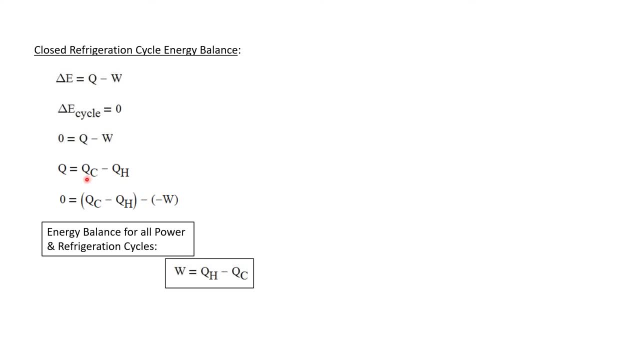 Now we've got to be careful about signs here. QC delivers energy to the cycle, so it will be taken as a positive, And we're going to add to that QH. but QH removes energy from the cycle, so it will be taken as a negative, And so we've got: Q is equal to QC minus QH. 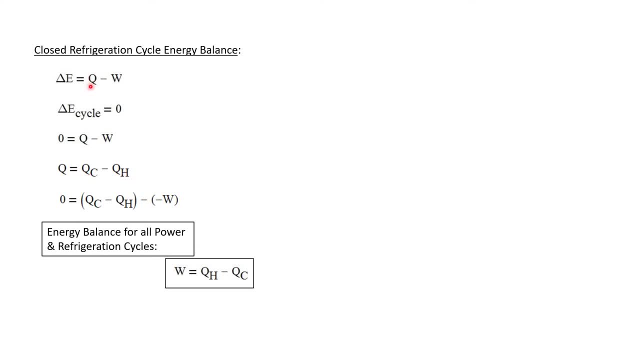 And we'll put QC minus QH in for Q in our energy balance. So we have 0 equals QC minus QH, and then we have this minus W. Okay, so W, though, is shown delivering energy to the system, and so it is taken as a negative, And so we're going to subtract a negative. 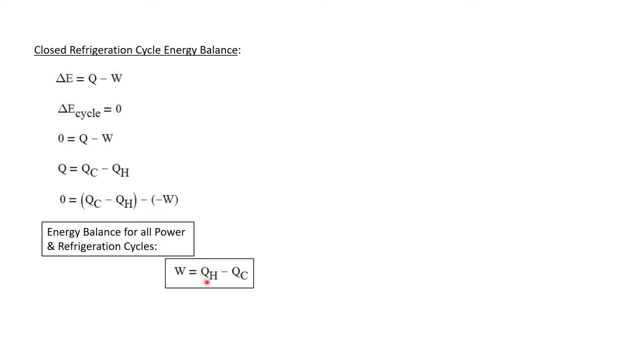 We can rearrange this as W is QH minus QC, And you may recall from our lesson that this is the same equation we got for a power cycle. so W is QH minus QC works for all power and refrigeration cycles. now we could have gotten the same. 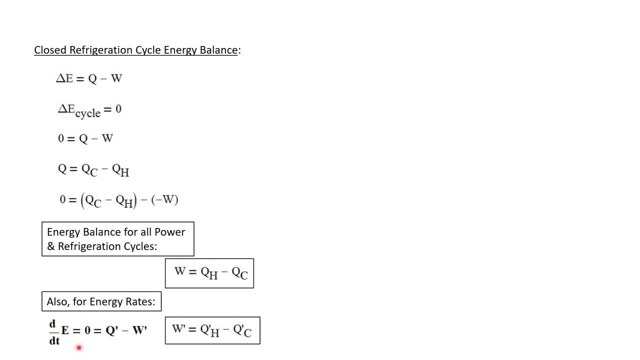 thing. if we had derived this equation for energy rates, we would have said: de DT is zero for a steady-state operation and that's equal to Q dot minus W dot. you know what? have gotten us to the same place: that W dot is equal Q dot, H minus. 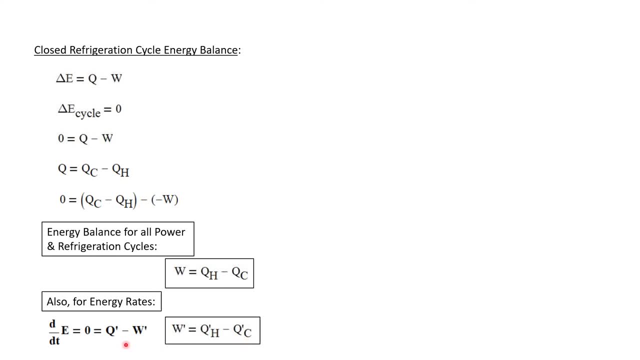 Q dot C. I'll leave this exercised to the student. our given data is that Q dot H was 0.6 kilowatts and W dot is 0.15 kilowatts, and our energy balance says that W dot is Q dot H minus Q dot C, and we want to solve this for Q dot C. 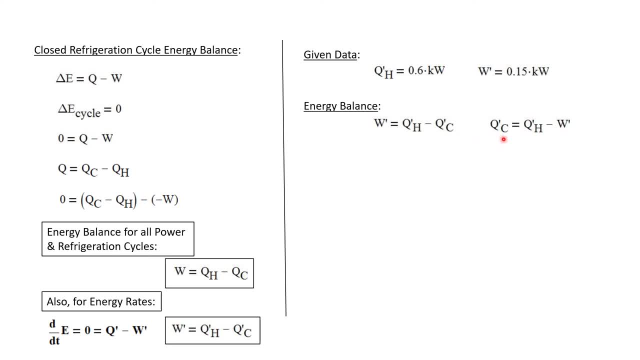 because that's our unknown- the rate of cooling from the refrigerated space. so Q dot C is Q dot H minus W dot. so solving for Q dot C, we get 0.6 kilowatts, which is Q dot H minus 0.15 kilowatts, which is W dot. we get Q dot C is 0.45 kilowatts. let's look: